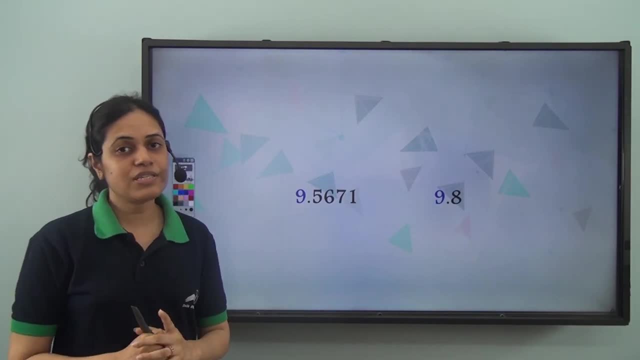 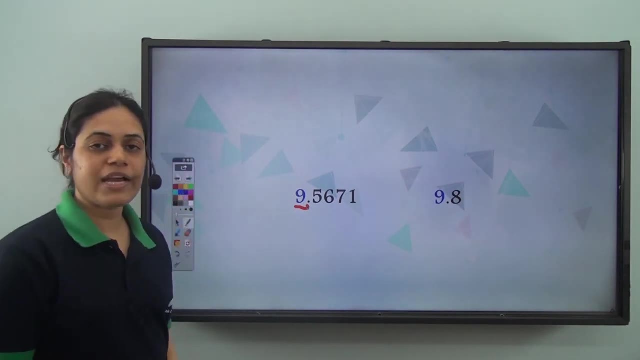 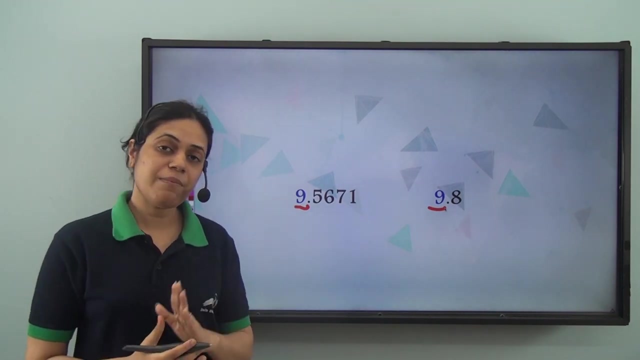 Now how do I compare these two numbers? So first I need to check the number before the decimal point. Now, over here, before the decimal point, I have 9 and in this case, as I have 9 before the decimal point, so both the numbers are equal. so what do I? 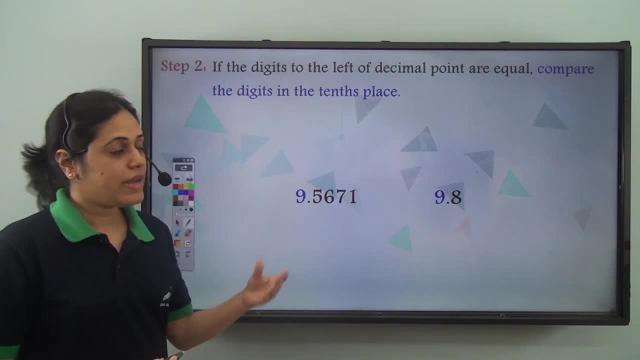 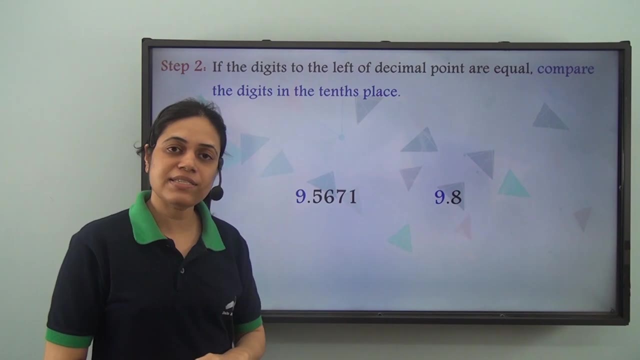 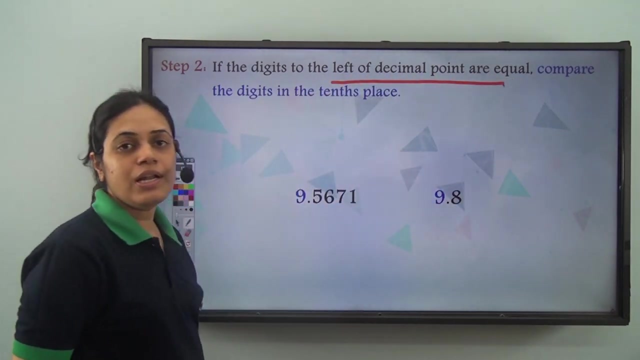 do next. so the next step. so in this case the number to the left of the decimal point is equal. in both the cases it is 9. then what do I do if the digits to the left of decimal points are equal? then compare the digits in the tens place. so 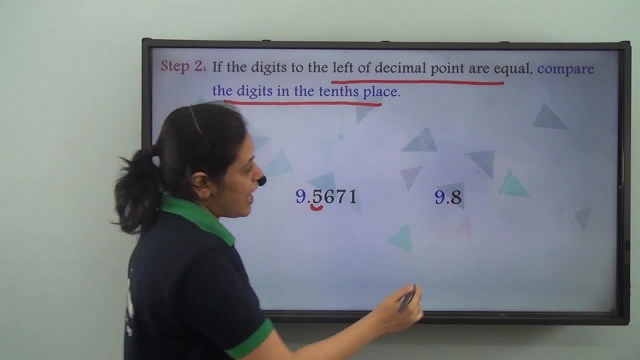 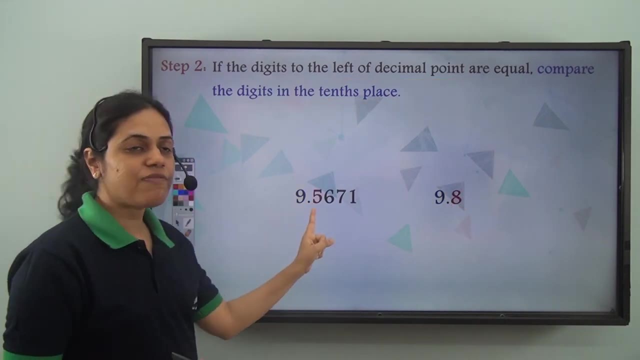 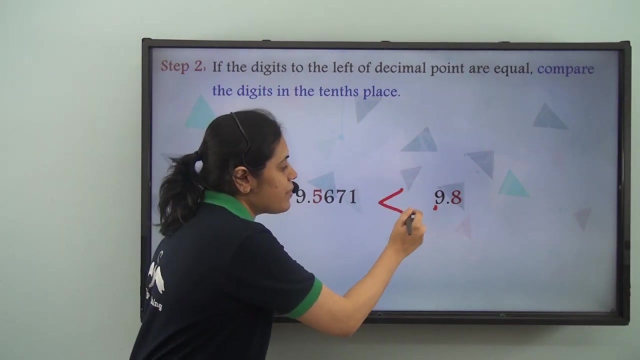 the tens place digit is 5 here and the tens place digit is 8 here, so I need to compare these two. so in this case it is 5 and in this case it is 8. no, which is greater? 8 is greater, so this number will be greater than this number. so 9.8 is. 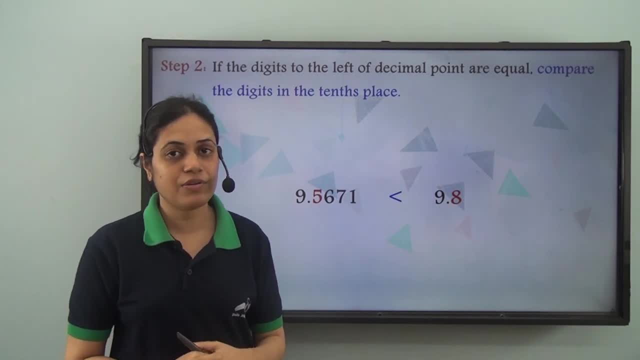 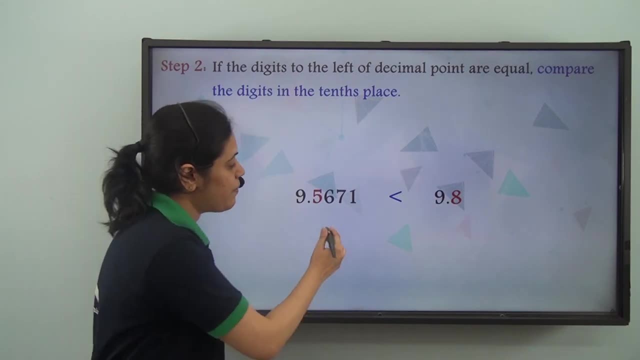 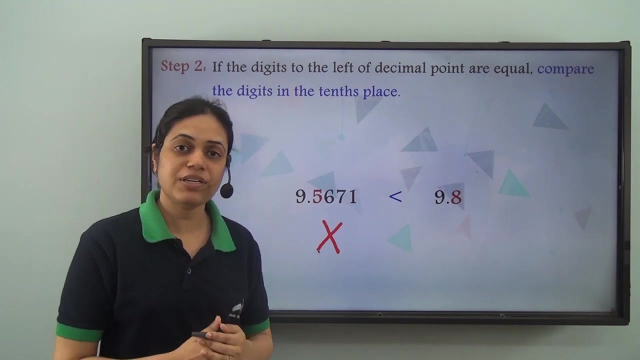 greater than 9.5671. so, although this number appears to be bigger because it has more number of digits, but it is not. So. in the case of decimal numbers, where we have digits after the decimal point as well, it does not matter how many digits. 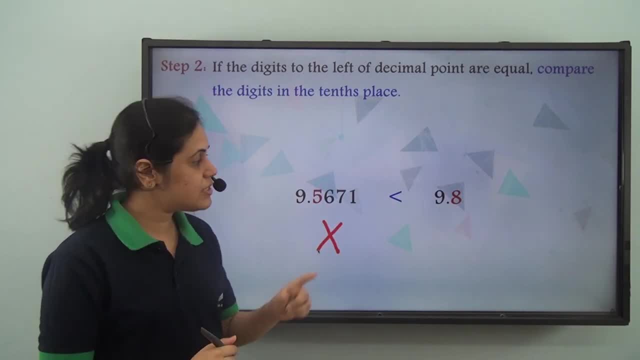 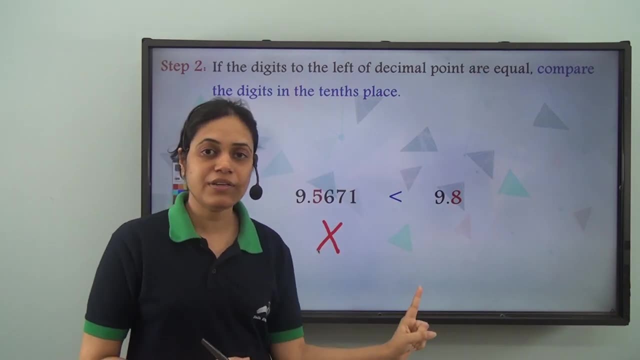 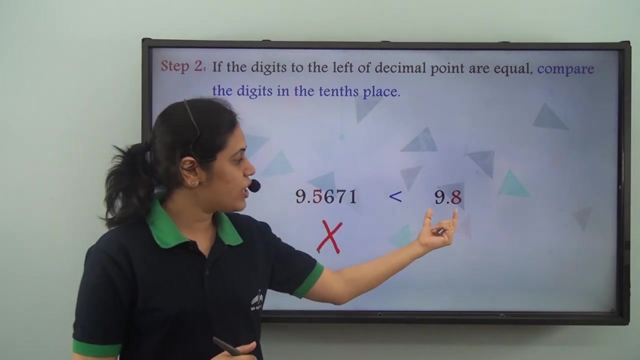 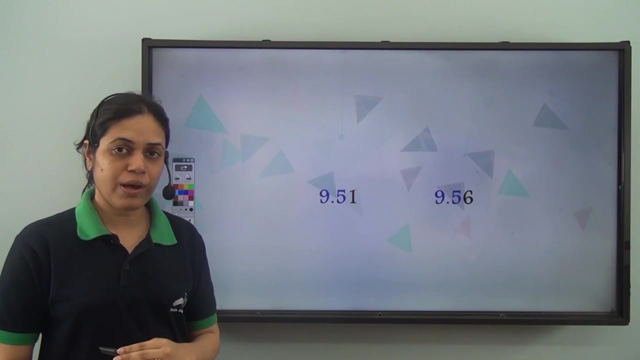 the numbers have. What we need to check is the digits in the tenths place in this case, and the number with the greater tenths place digit is greater. So 8 is greater than 5.. So 9.8 is greater than 9.5671.. Now, what about these two numbers? In these two numbers, the 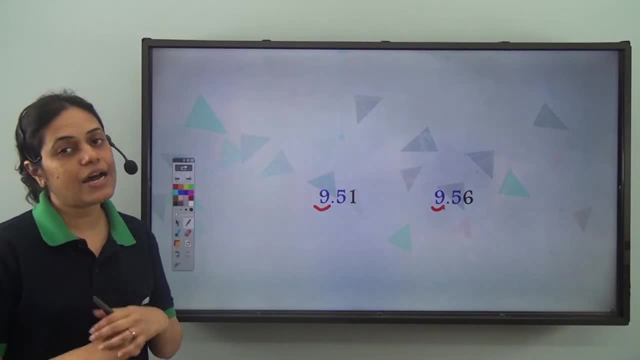 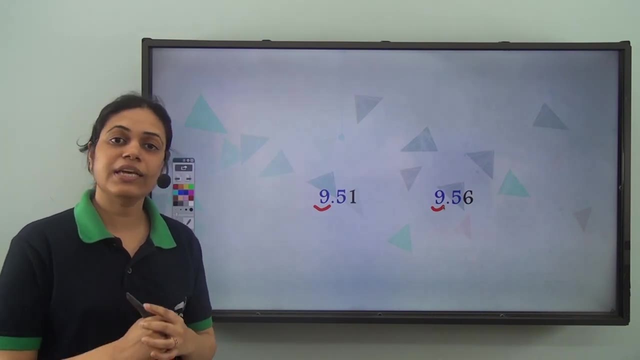 digits to the left of the decimal point are equal, So 9, 9- they are equal. Next, I need to look at the digits in the tenths place. Over here I have 5 in the tenths place and in this case as well. 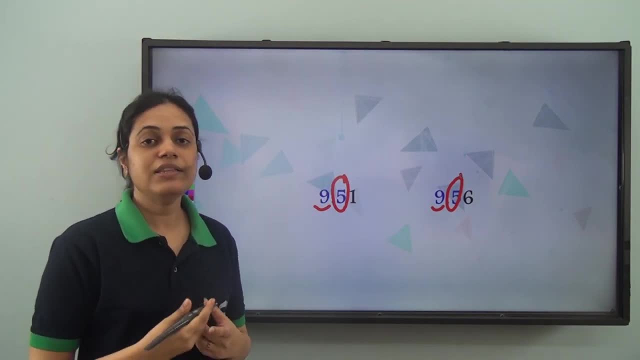 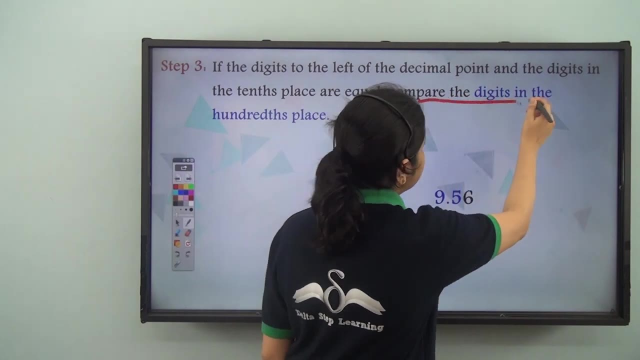 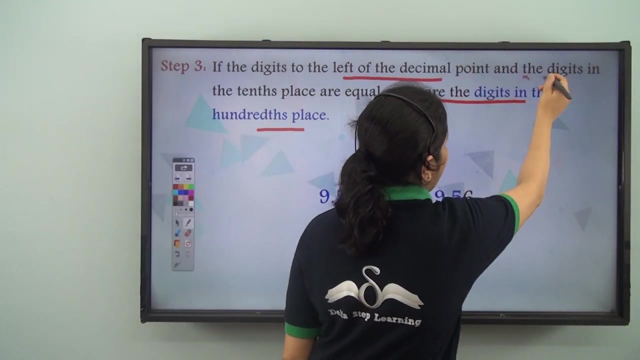 I have 5 in the tenths place. So once again, the digits in the tenths place are equal. So the next step is to compare the digits in the hundredths place. So if the digits to the left of the decimal point and the digits in the tenths place are equal, then we move on. 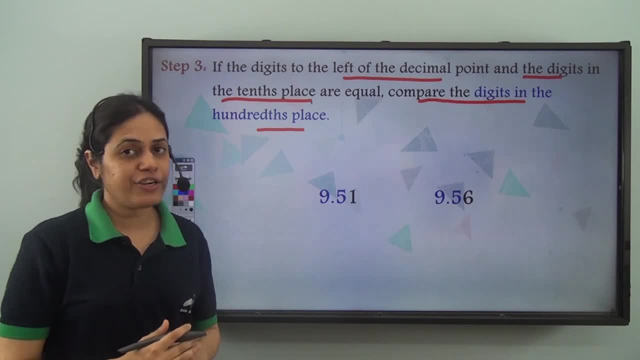 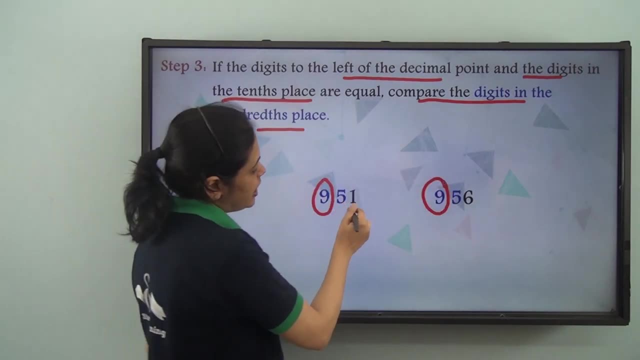 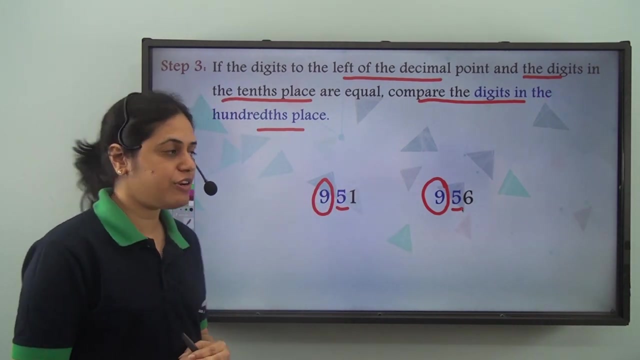 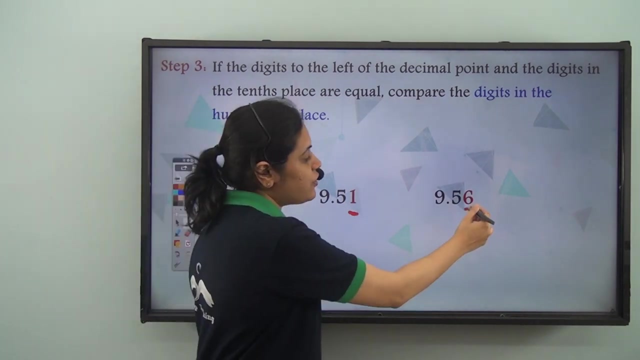 further to the right, that is, to the hundredths place. So we check the digit before the decimal point, We check the tenths place. They are equal. So we move on to the next place, which is the hundredths place. In this case the hundredths place is 1 and in this case the hundredths place 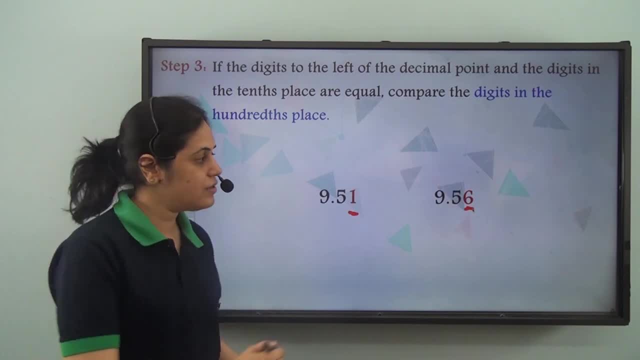 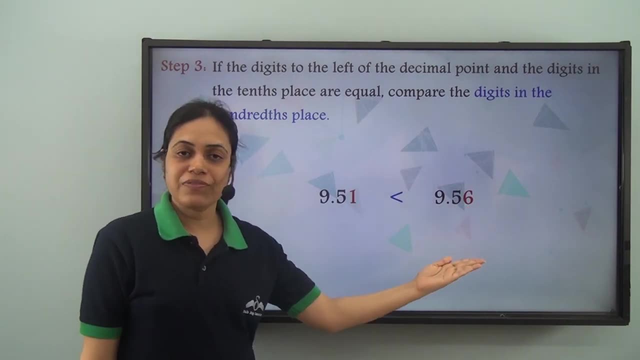 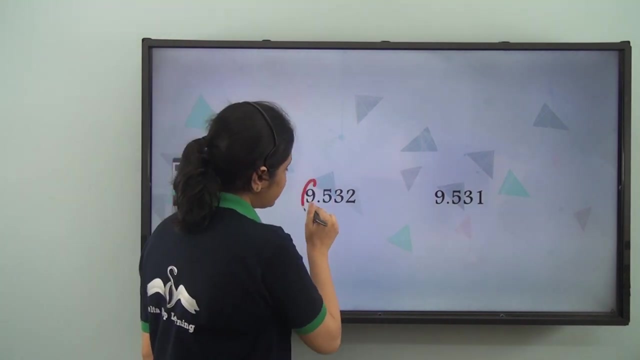 is 6.. Now, 6 is greater than 1.. So this number is greater than 1.. This number is greater than this number. So I can say 9.56 is greater than 9.51 or 9.51 is less than 9.56.. Now, what about these two numbers In these two numbers? first I check. 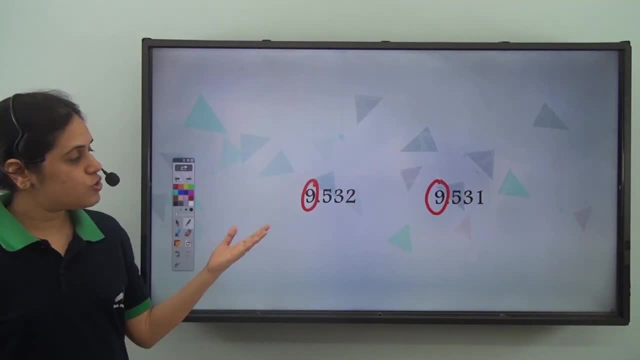 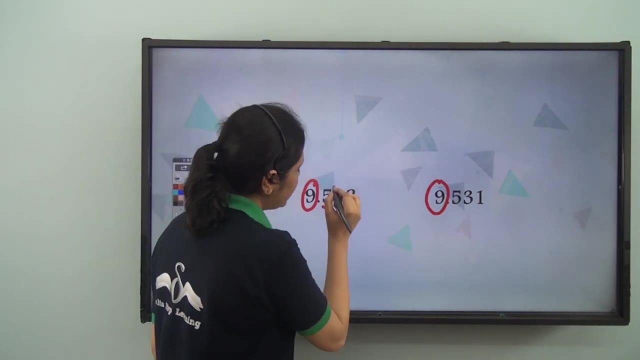 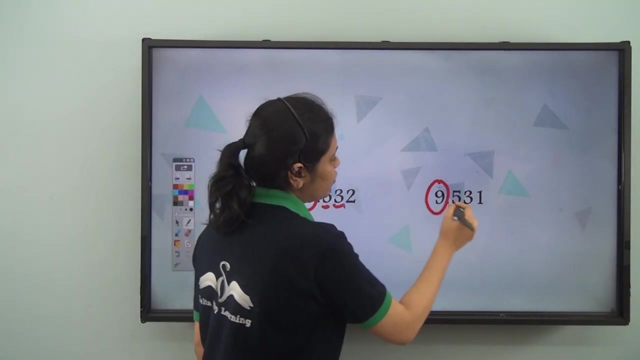 the digits to the left of the decimal point. So in both the numbers they are 9.. So 9 is equal to 9.. Next I go To the tenths place. The tenths place digits are also equal: It's 5.. Next I go to the hundredths. 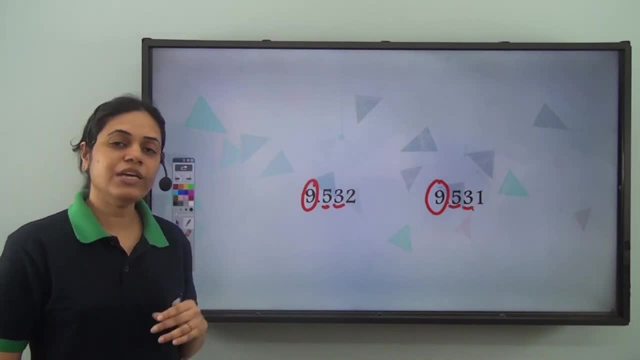 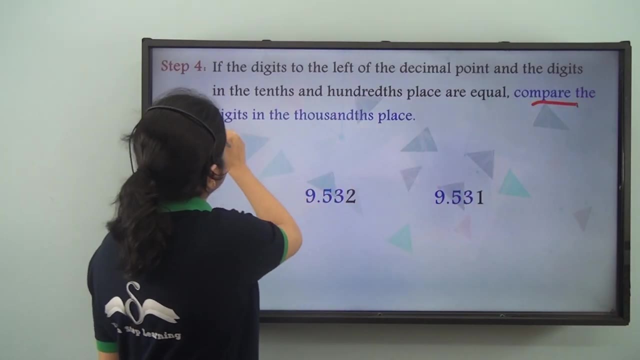 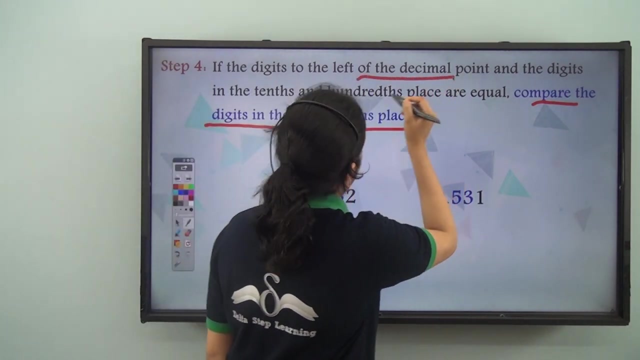 place. The hundredths place digit is 3 in each of the cases. So next I need to compare the digits in the thousandths place. So if the digits to the left of the decimal point and the digits in the tenths and the hundredths place are equal, So I can say 9.56 is greater. 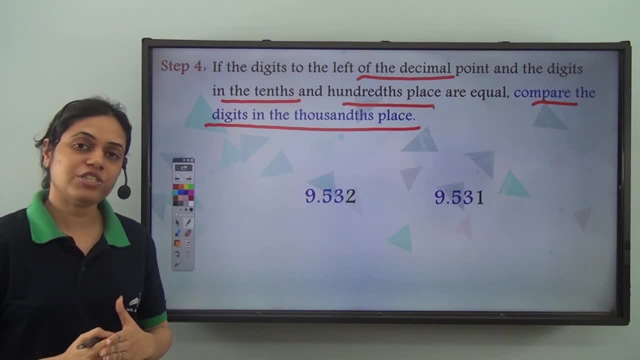 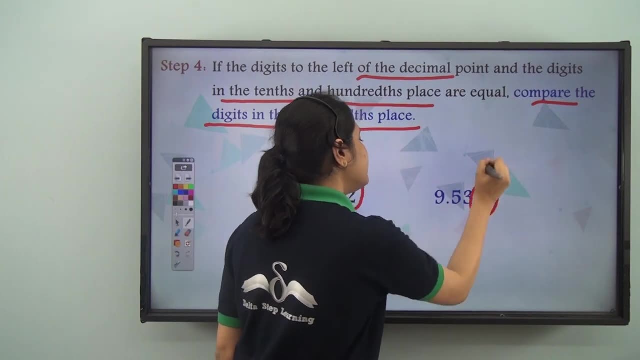 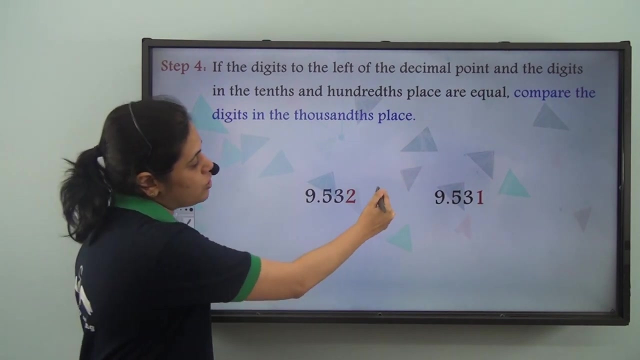 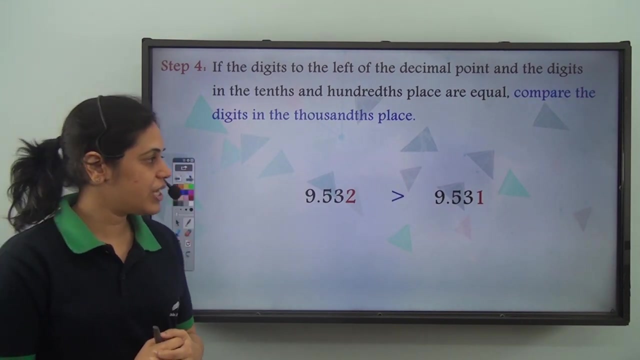 than 1.. Then I need to compare the digits in the thousandths place. So over here it is 2 and here it is 1.. 2 is greater than 1.. So this number is greater than this number. So 9.532 is greater. 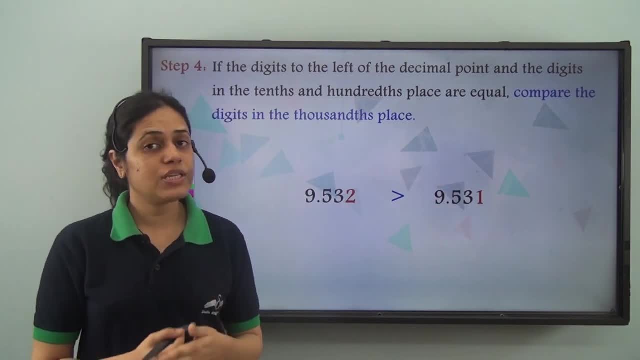 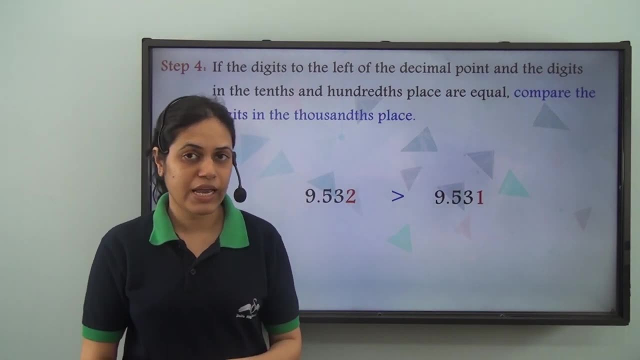 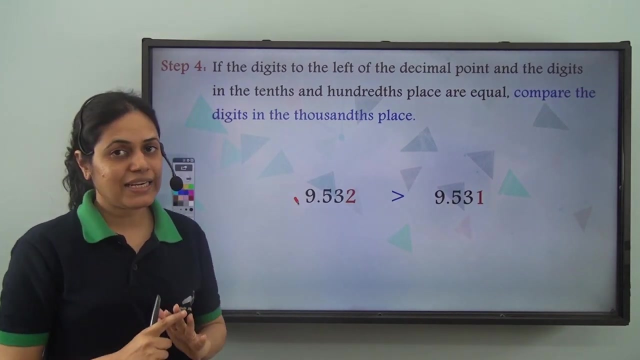 than 9.531.. So this is how I can compare 6.. the decimal numbers: We keep on moving further to the right. So first thing is to check the digits before the decimal point. In that case we compare the number as a whole and the decimal number which. 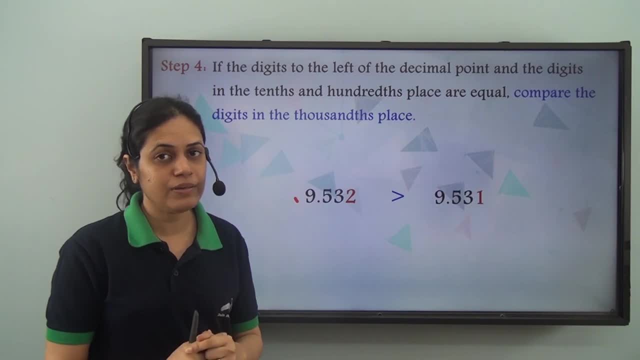 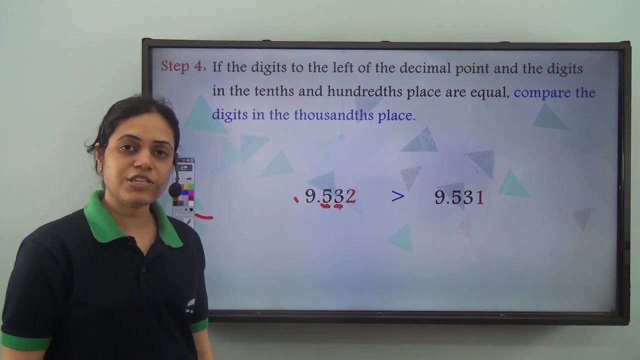 has a greater number to the left of the decimal point will be bigger. Now if the numbers, that is the digits to the left of the decimal point, are equal, then we first check the tens digit. If they are equal, then we compare the hundreds digit. If they are equal, then we compare the thousands. 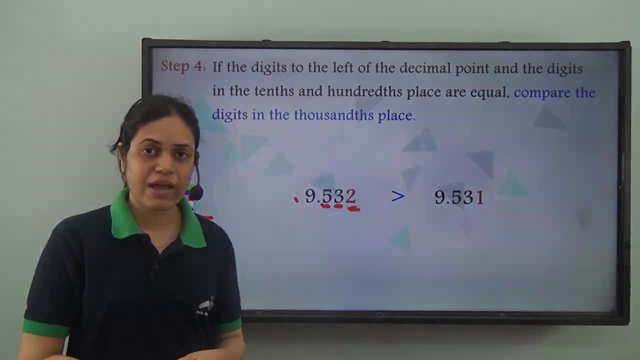 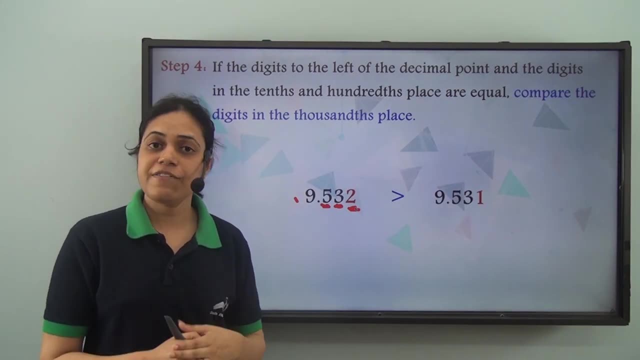 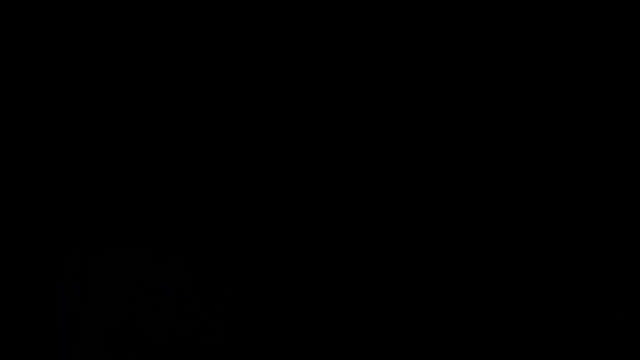 digit and we keep on moving in this manner till we get a place in which there are unequal digits. Also, if there are no unequal digits, then we can say that the two numbers are equal. If you like this video, then subscribe to our channel. You can also register for free at: 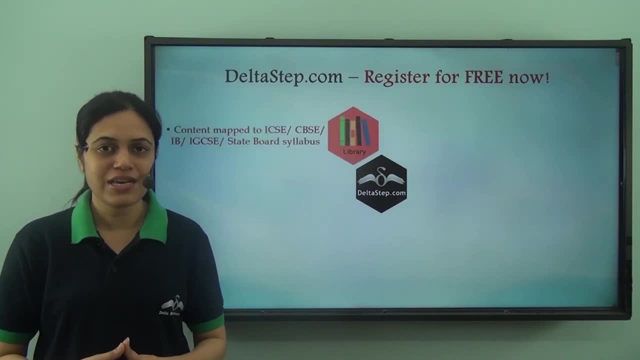 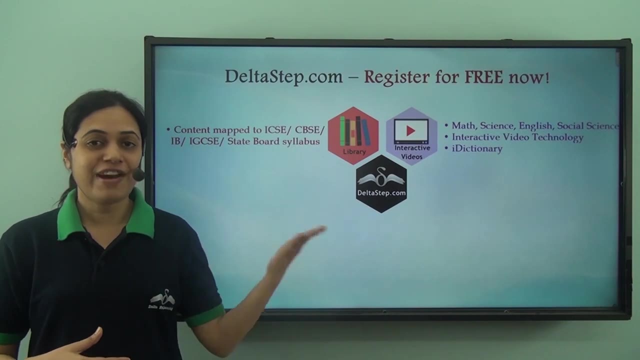 deltastepcom to get all the learning resources as per CBSC, ICSC, IB, Cambridge or any other curriculum. Over 5000 amazing lectures on Maths, Science, English and Social Science. Our unique interactive video technology keeps you engaged and our iDictionary feature allows you to. 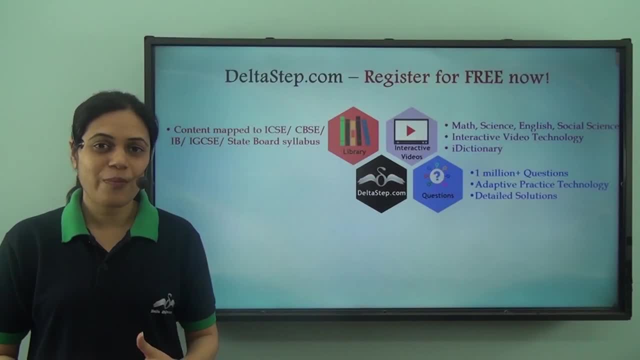 quickly revise any concept. Master each topic at your own pace with our adaptive practice technology and 1 million plus questions. Get instant answers and detailed solutions. Be exam ready by taking unlimited mock tests. performance analysis along with actionable feedback. Personal tutors to resolve. 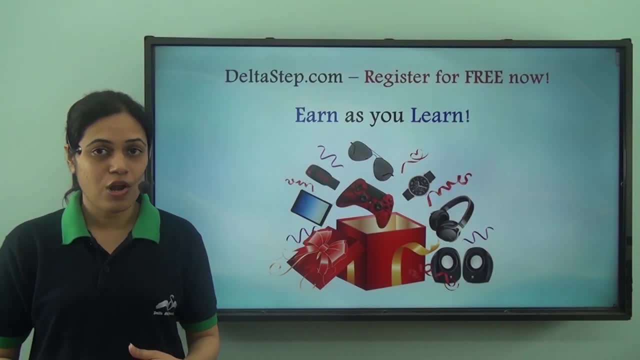 the slightest of your doubts. And that's not all. you can also win exciting prizes like PlayStations, iPads, watches and many more, along with certificates through our earn as you learn program. So at deltastepcom, learning is not just fun and easy. it is rewarding too, So register for free now.